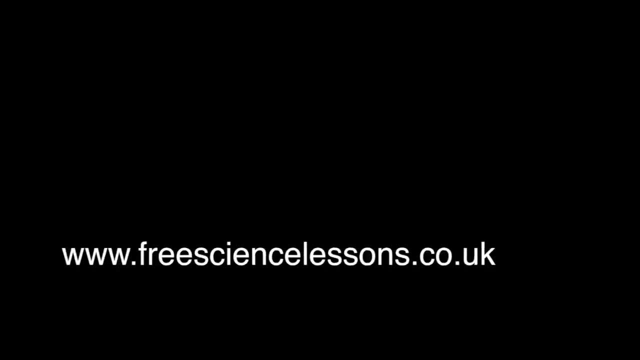 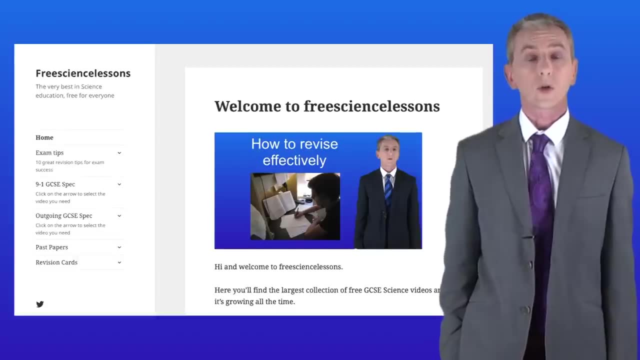 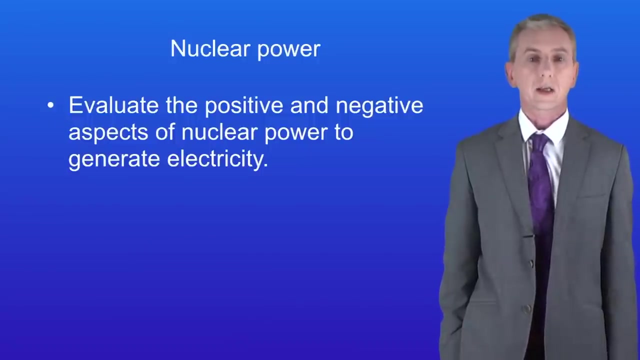 Hi and welcome back to freesciencelessonscouk. By the end of this video you should be able to evaluate the positive and the negative aspects of nuclear power to generate electricity. I'm showing you here a nuclear power plant in England. Now, the first key idea about nuclear power is that 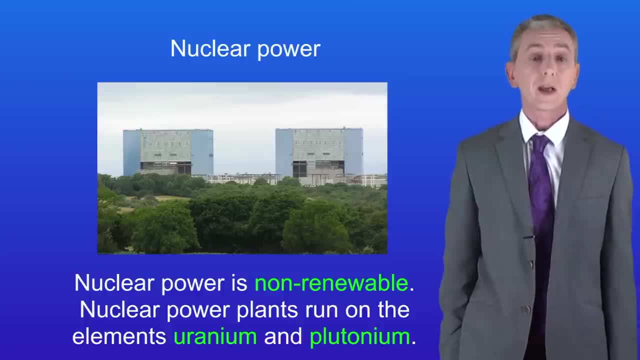 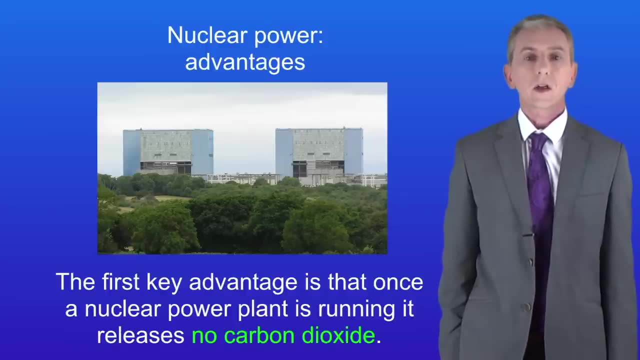 it's non-renewable. Nuclear power plants run on the elements uranium and plutonium. Let's take a look at the advantages of generating electricity by nuclear power. The first advantage is that once a nuclear power plant is running, it does not release carbon dioxide. That means that nuclear 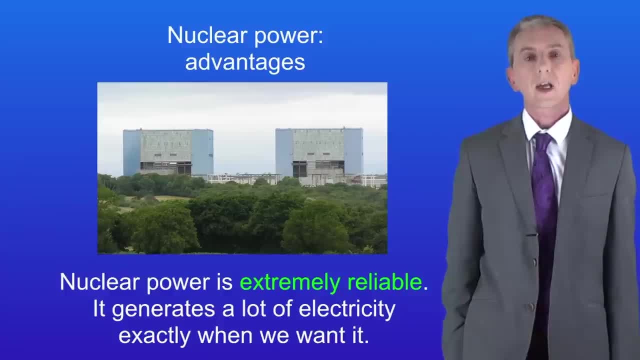 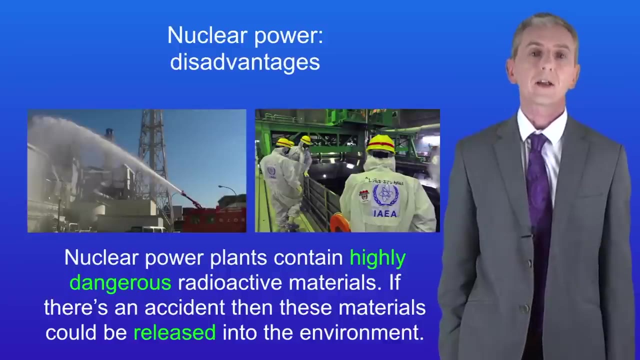 power does not contribute to climate change. Here's the second advantage. Nuclear power is extremely reliable. It generates a lot of electricity exactly when we want it. Now there are some disadvantages to nuclear power. The first is that nuclear power plants contain highly dangerous radioactive materials. Now that means that if there's an accident, then these materials 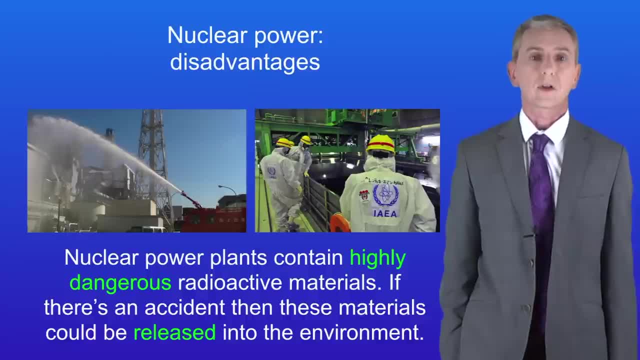 can be released into the environment That could be potentially disastrous. I'm showing you here a Japanese nuclear power plant. In 2011, a tsunami flooded the power plant and that caused the release of radioactive material. Over 150,000 people who live nearby had to be evacuated, and 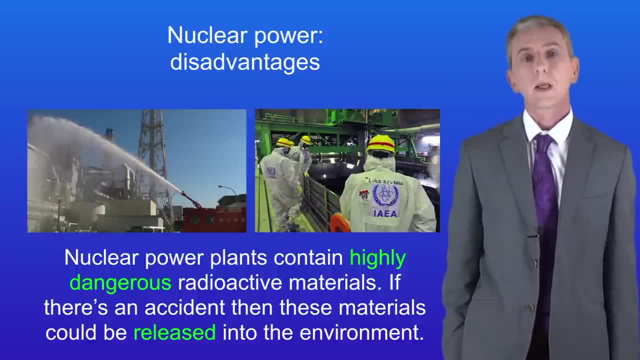 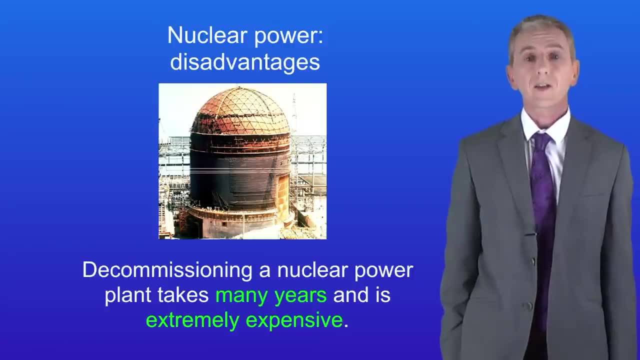 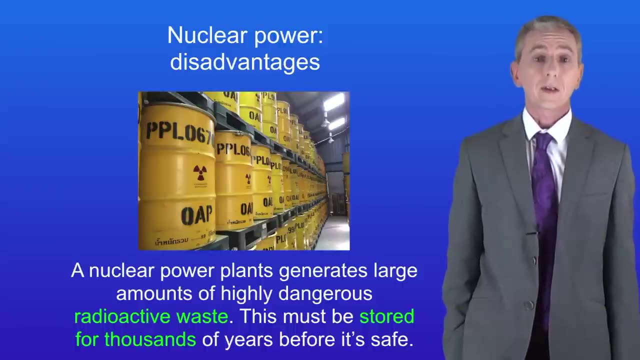 the cleanup will continue for many years. Here's the second disadvantage. At the end of its life, a nuclear power plant has to be decommissioned or dismantled. That takes many years and it's extremely expensive. Here's the third disadvantage. During its life and after decommissioning a nuclear 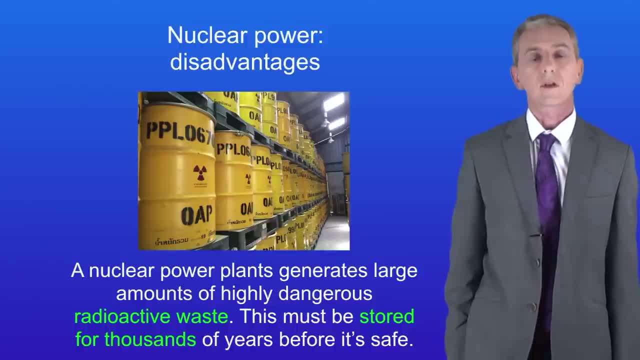 power plant generates large amounts of highly dangerous radioactive waste. That waste has to be stored for thousands of years before it's safe. Now in the next video, we're going to be exploring how different power plants, including nuclear, will contribute to the UK's energy use in the future. 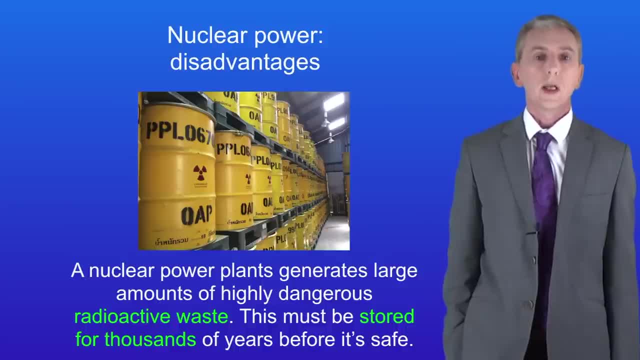 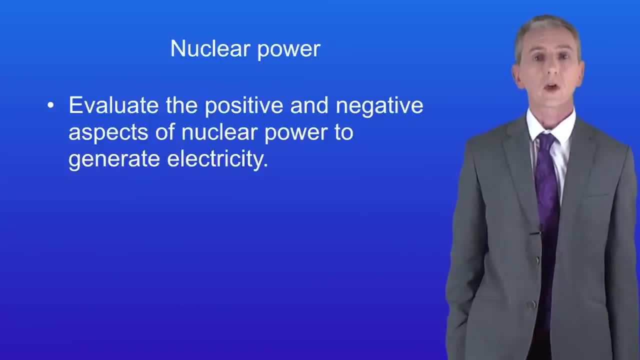 Remember, you'll find plenty of questions on nuclear power in my revision workbook and you can get that by clicking on the link above. Okay, so hopefully now you should be able to evaluate the positive and negative aspects of nuclear power to generate electricity.